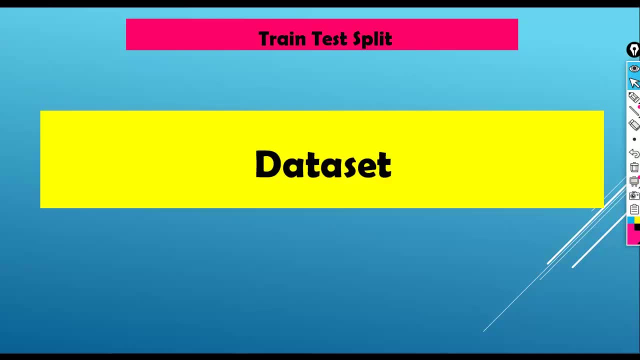 are dividing our data set into two subsets, One for training and one for testing, So common split percentages are: we can keep 80% data for training purpose and we can keep 80% data for training purpose, So we can keep 80% data. 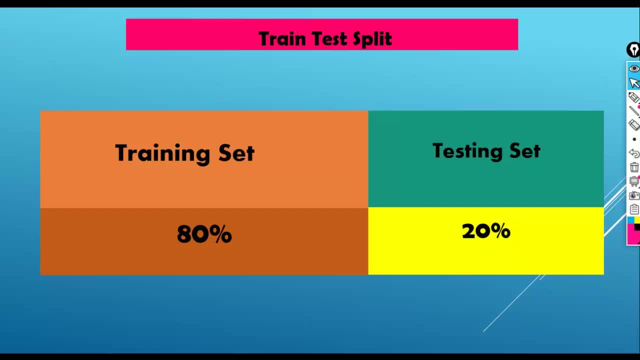 for training purpose and we can keep aside 20% data for testing purpose. We can use 67% for training purpose And we can keep aside thirty three percent data for testing purpose. Also, we can use 50 percent data for training purpose. Same. 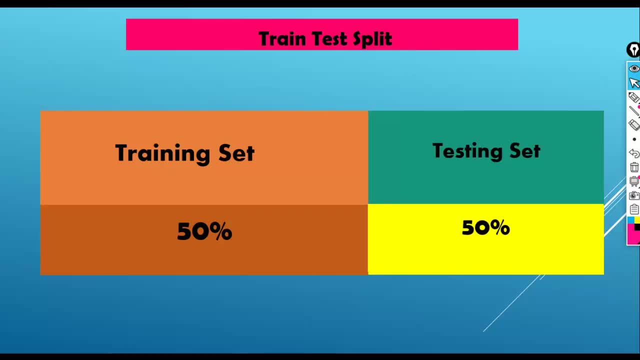 50% data we can keep aside for testing purpose, But the most common split percentage is 80% and 20%. So we can use 80% data for training purpose and we can keep aside 20% data for testing purpose. so please remember this percentage is. 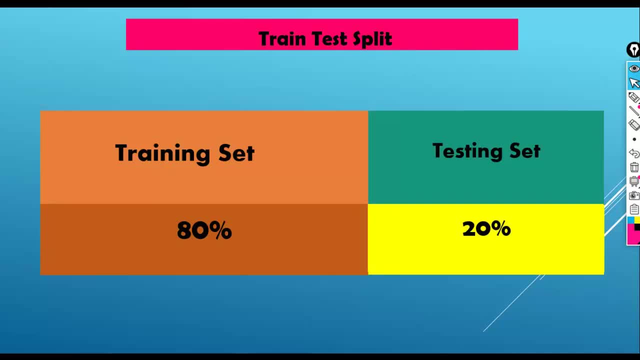 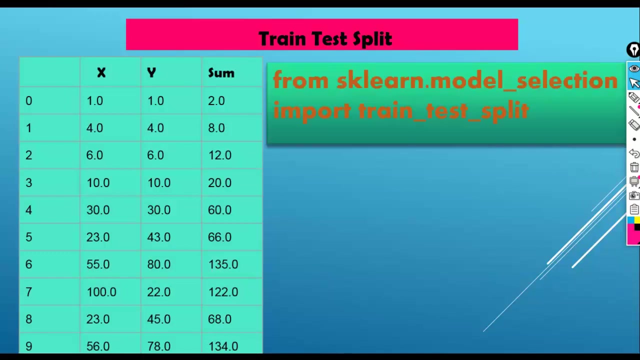 totally depend on the size of your data set, but the most common splitting percentage is 80: 20. so we can use 80% data for training purpose and we keep aside 20% data for testing purpose. so for this we can use train test split module of sk learn that we can import like from sk learn dot. 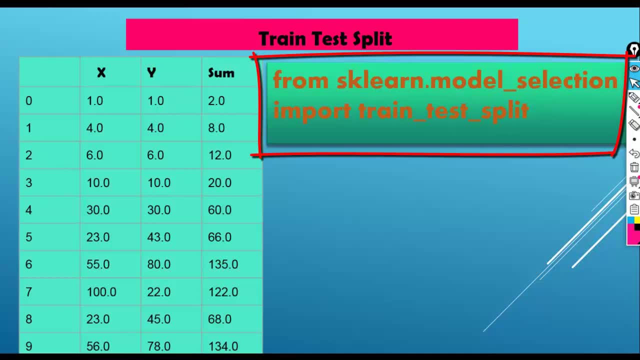 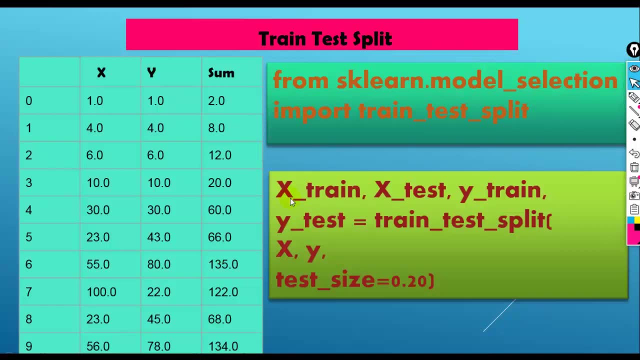 model underscore selection. we can import train underscore test underscore split. so this train test split divides our data into four parts: one independent and dependent pair of training set and one independent and dependent pair of testing set. as you can see here, test underscore size is equal to 0.20, means we are keeping aside 20% data for testing purpose that you can see over here. 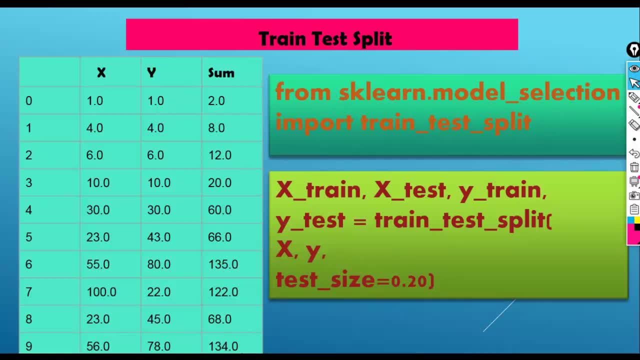 as i said, this train test split divides our data into four parts. this is x train, x train and this is y train. so this part is x train, our independent variables of training set, and here y train, our dependent variables of training set. so this is our training set. so this is our testing set, as you can see here. 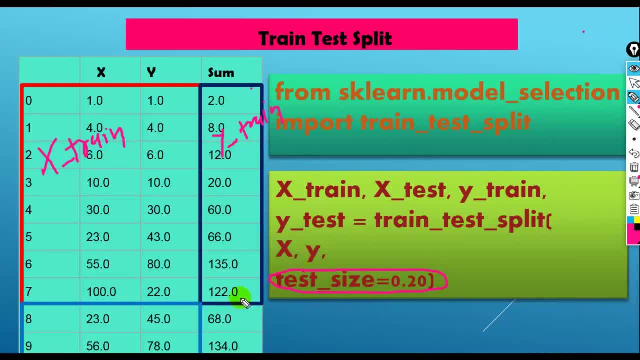 we kept aside 20% data for testing purpose. you can see over here total. we are having 10 samples. we keep aside 20% data for testing purpose. that you can see over here two samples out of 10 samples, 20% data. so this is our testing set and 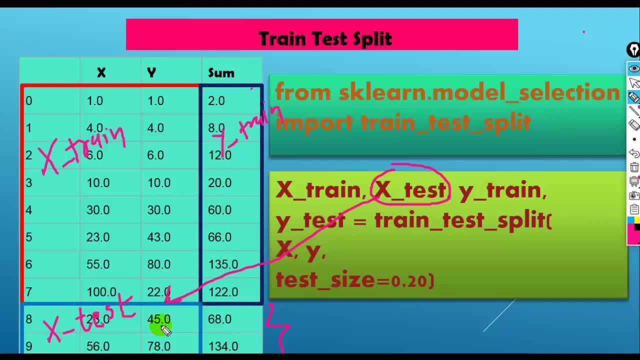 this is x test- independent variables of testing set. and this is y test- y underscore test- dependent variables of testing set. so this way, train test split divides our data into four parts: x train, y train, x test and y test. so we can consider: this is our training set and this is. 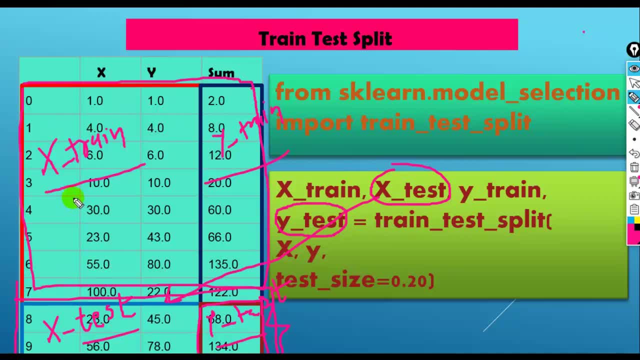 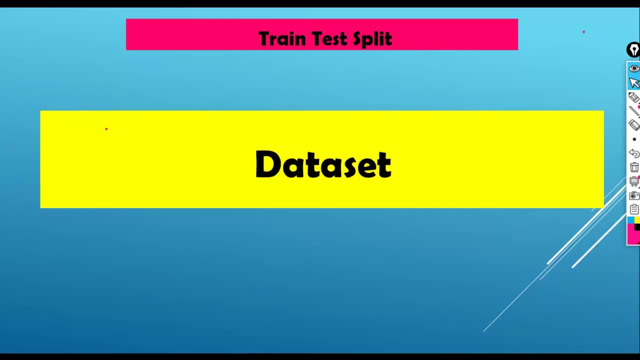 our testing set. so training set with pair of independent variables and dependent variables and testing set with independent variables and dependent variables. So, as I said, in train test plate we are dividing our data set into two subsets, one for training and one for testing. and further train test plate divides our data into four parts. 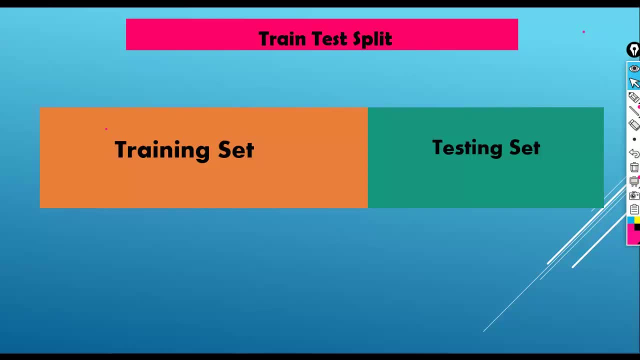 So two parts of training set and two parts of testing set. So our training set is divided into X train and Y train and our testing set is divided into X test and Y test. So our train test plate divides our data into four parts: X train, Y train, X test and Y test. 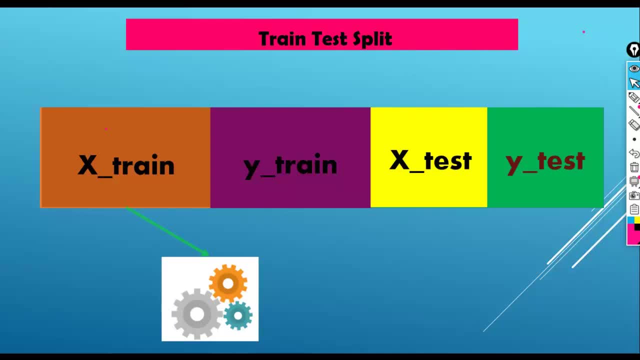 So we are going to train our machine learning algorithms on X train and Y train, Our training set, and we will perform our prediction using X test, Our unseen samples that we kept aside for testing purpose, and we will compare our predicted result that we have stored. 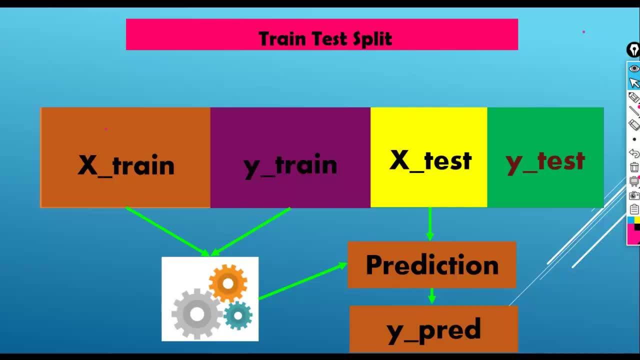 in Y test and Y test, Y underscore pred, which is an identifier. You can use any other name. So we are storing our predictions into Y underscore pred and we will compare our predicted result by our model with Y underscore test. So at the end we are comparing our predicted result with actual result. 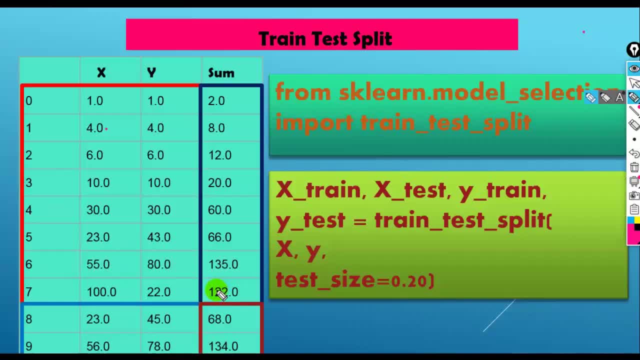 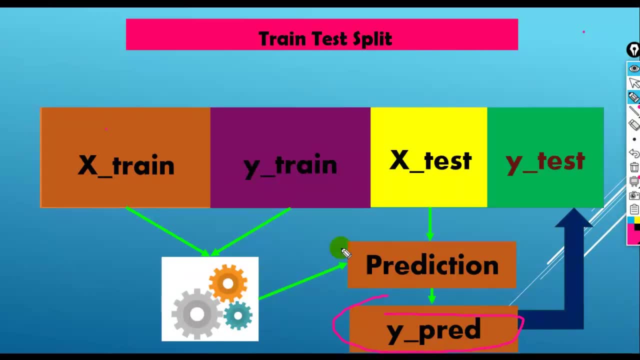 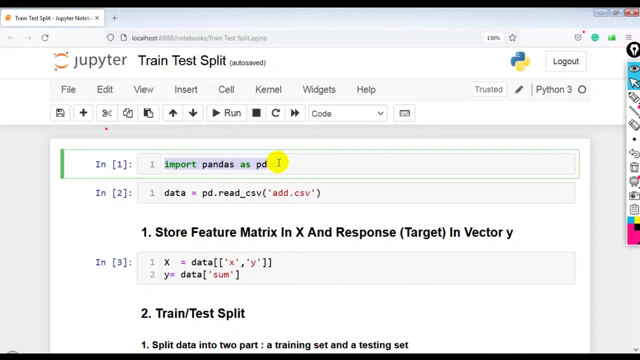 that we have stored inside Y underscore test- This one, our actual results that we will compare with predicted results By our model. So let me show you one simple example of train test plate. So let's jump to Jupyter Notebook. So, as you can see here, I have imported Pandas as PD. 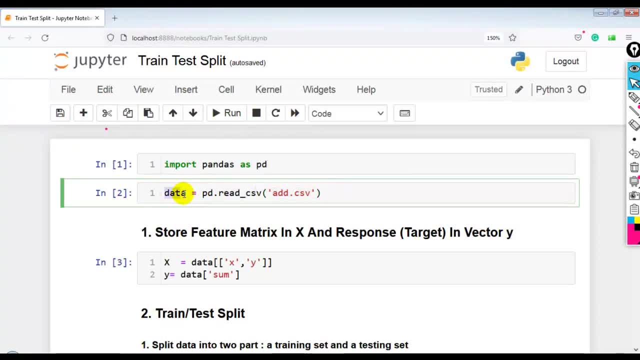 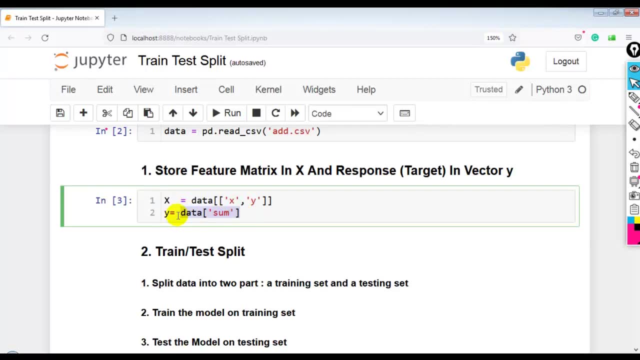 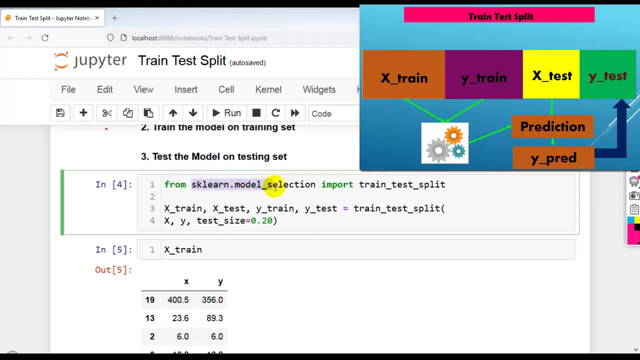 and here we are loading our data set as Pandas data frame, and here I have stored independent variables into X and our dependent variable sum into Y. Now our train test plate. So for that we have to import from sklearnmodel underscore selection, We have to import train underscore test, underscore split. 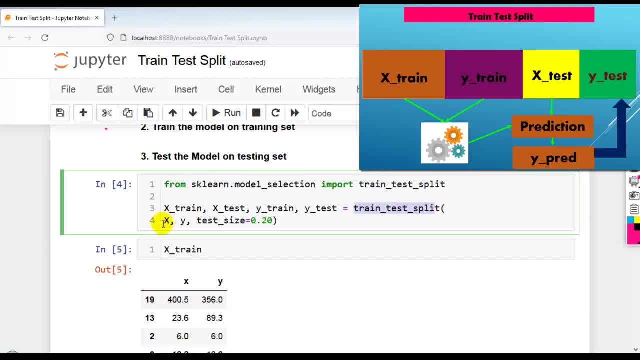 and this is our train underscore test, underscore split. Here you can see our independent variables and our dependent variable sum, and here I have set test size with parameter test underscore size is equal to 0.20.. We are keeping aside 20% data for testing purpose. 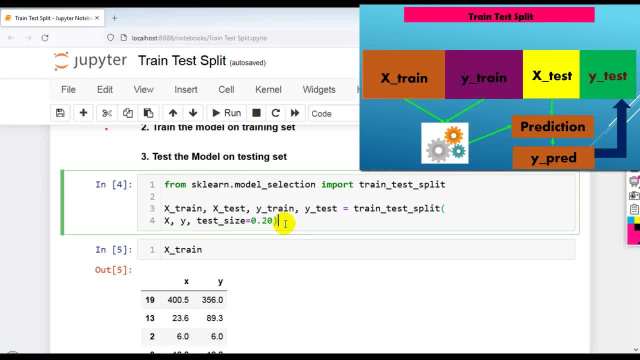 And, as I said, train test split divides our data into four parts: One for training and one for testing. That you can see over here: X underscore train, X underscore test, Y underscore train and Y underscore test. So we are going to train our model on X train and Y train on our training set. 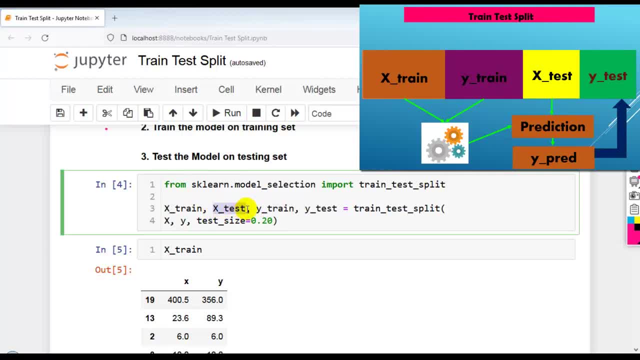 and we will perform predictions using X test, our unseen samples, and we will compare our predicted result by our model with Y test. So Y test contains our actual result. So this way we can use train test split of sklearn, scikit-learn. Let me execute this cell. 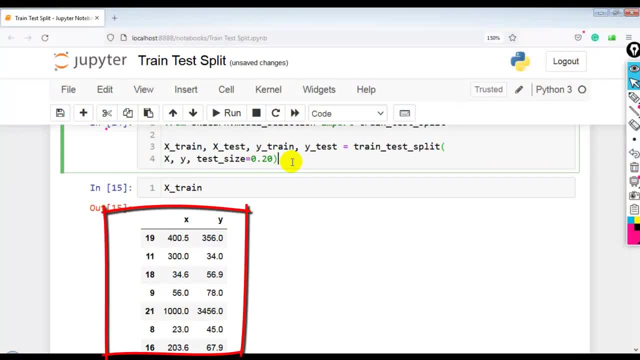 As you can see here, this train test split, generating random samples at every run that you can see over here from our data set. So if you want same split as mine, then here we have to use another parameter, random underscore state, and you can set it to any number. 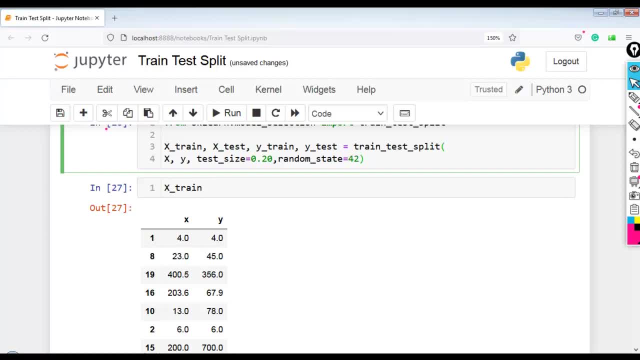 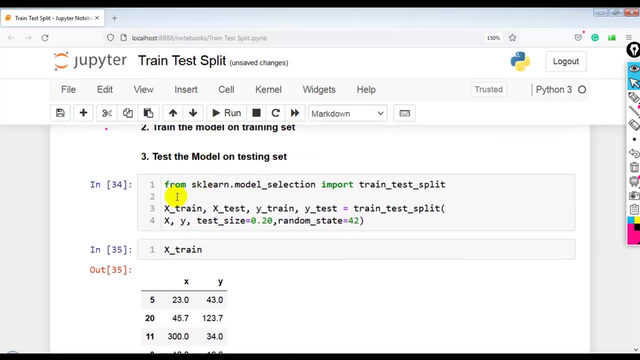 Let me set it to 40.. So if you are using 42, then we get same split that you can see over here at every run that you can see over here. So this way we can use train test split for model evaluation. So here I have used linear regression model. 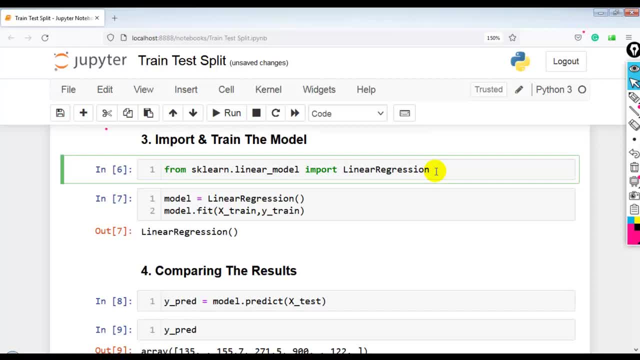 You can use any other regression model, because this is a regression problem, right? Because our target variable is continuous. to use linear regression Here, I have imported from sklearn dot linear underscore model, Import linear regression. Let me execute this cell As you can see here. 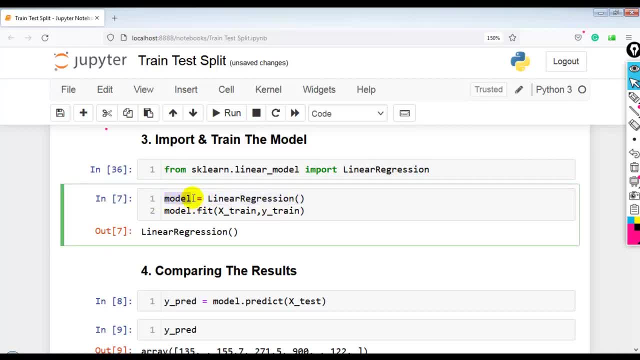 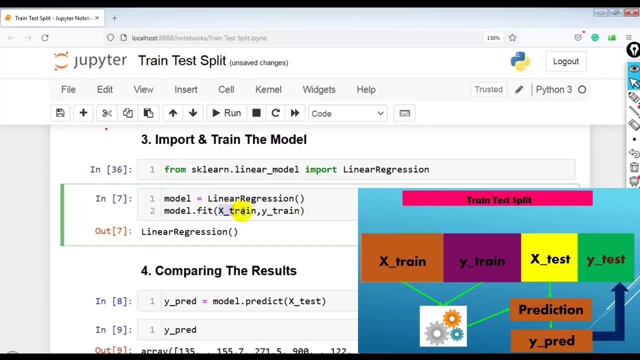 I have created instance of this model linear regression and fit method, model dot fit to train our model linear regression on our training set, X train and Y train. Set of independent and dependent variables of training set. Let me execute this cell As you can see over here. 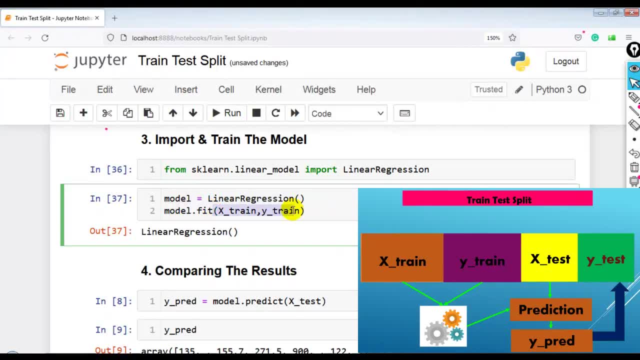 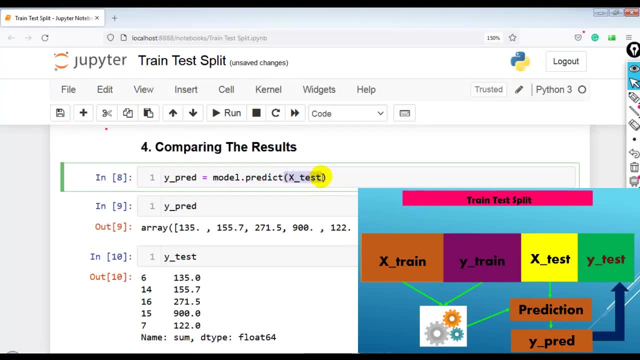 now our model is successful, Successfully trained on our training set, As you can see over here. model dot predict. As I said, we are going to perform prediction using unseen samples available inside X underscore test and I have stored predicted results by our model into Y underscore pred. 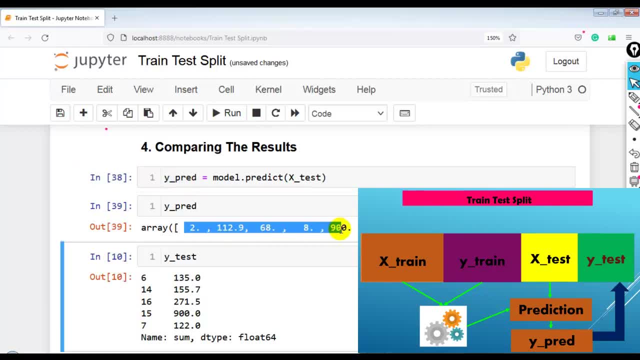 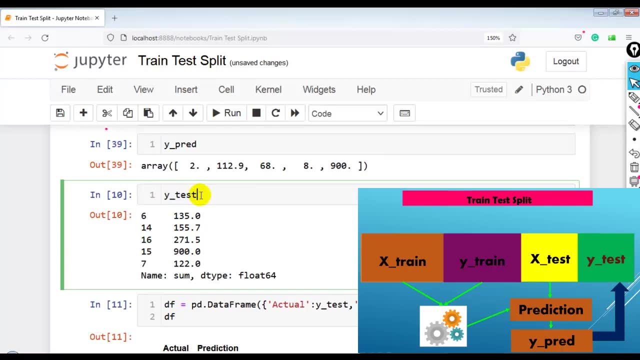 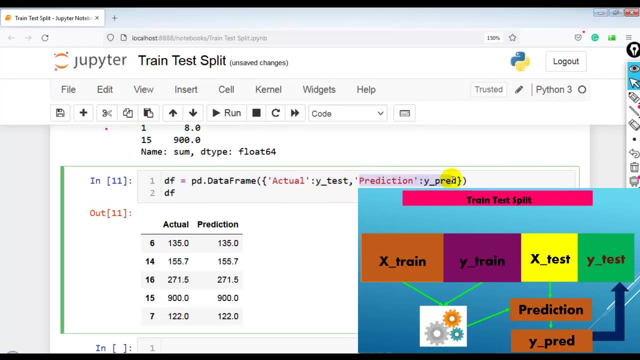 Let me execute this cell. As you can see over here, predicted results by our model linear regression And as you can see over here, Y underscore test our actual results. And here I have created data frame to compare actual results with predicted results. Let me execute this cell. 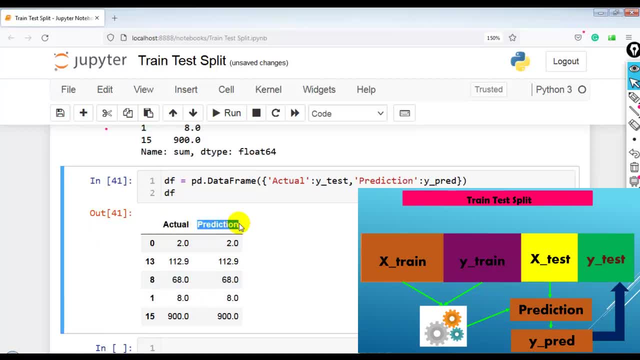 As you can see over here, our actual results and predicted results by our model. So this way we can use train test split to evaluate the performance of our machine learning algorithms. So now let's revise train test split. So this is our data set. 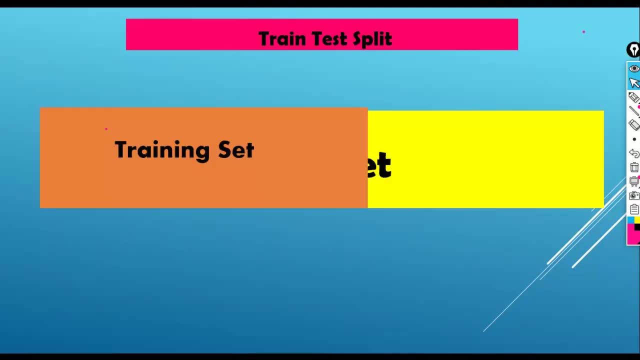 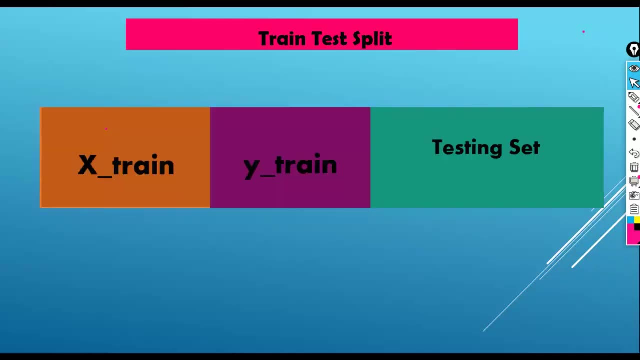 Train test split divides our data set into two set: training set and testing set, And training set further divided into two parts: X train, Y train And testing set further divided into two parts: X test and Y test. So we are going to train our machine learning algorithms on X train and Y train. 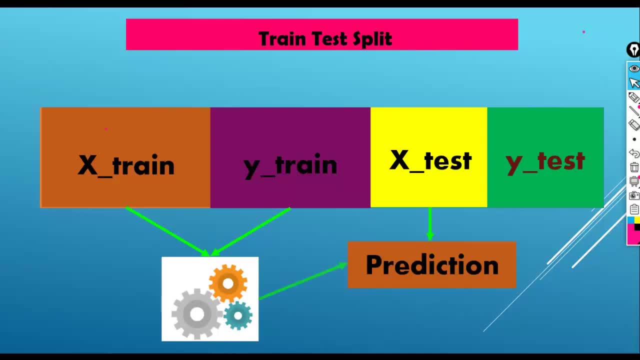 And we will perform predictions using X test, our unseen samples, And we will store our predicted results into Y underscore pred And we will compare our predicted results available inside Y underscore pred With our actual results available inside Y underscore test. So this way we can use train test split to evaluate the performance of our machine learning. 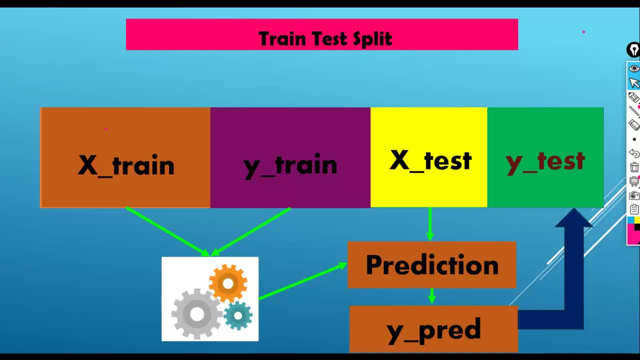 algorithms. Hope you like this video. Please don't forget to subscribe this channel. If you like this video, smash that like button. Thank you very much for watching this video. Take care, Bye, bye, See you in the next video.